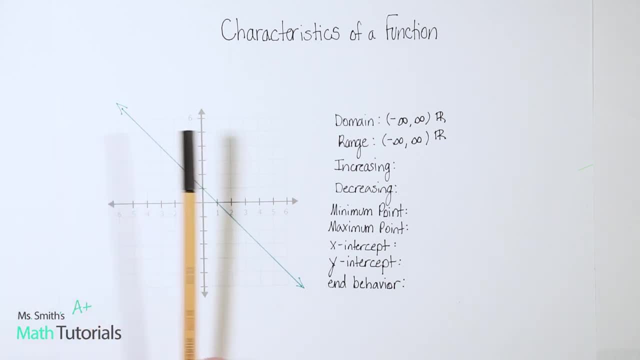 important thing is that we read this graph left to right, always just like a book, So left to right. So looking at this graph, reading it left to right, I see that we're moving down. It's kind of like going down a roller coaster. So this graph does not increase at all When we want to know an interval. 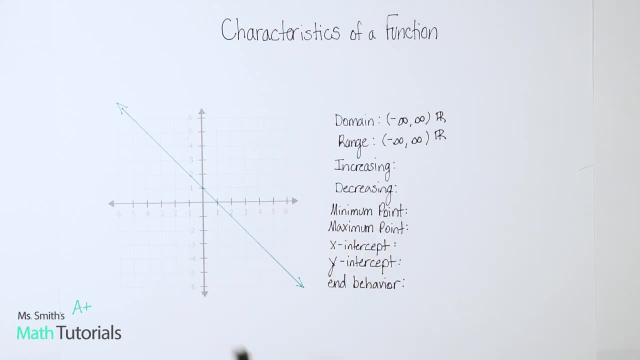 of increasing. it's going to be negative infinity to positive infinity. So we're going to want to know an interval of increasing. it's going to be negative infinity to positive infinity. In this particular case, there is none. It's not increasing at all and it's not going to increase. So we would just put. 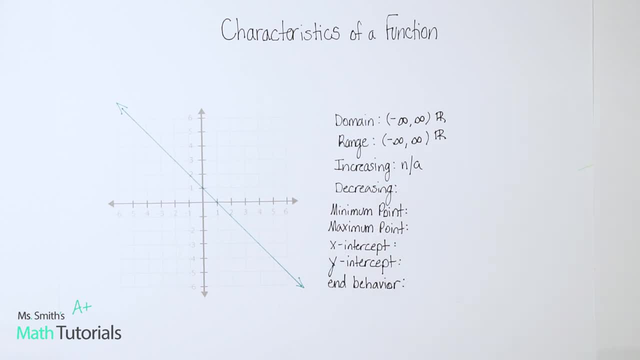 n, a, or you could put none. Don't put zero, because that zero is a number, but you just want to put that it's. there is none Decreasing. Yes, we are decreasing from here all the way to the end of the graph and we will be decreasing for infinity. So we want that interval of time based on the x-axis. 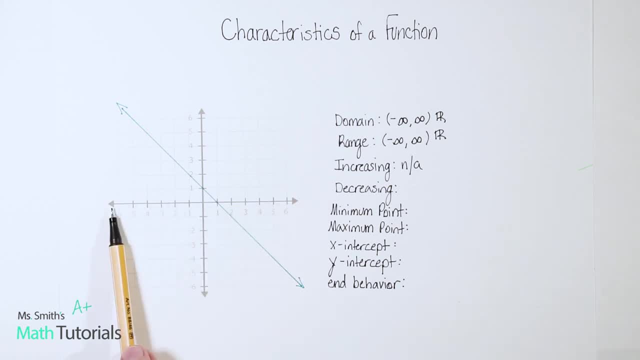 when we are decreasing. So in this case, looking at the x-axis now, some people would say, oh, that falls at negative six. Well, no, that's just where the arrow is shown. but that arrow indicates that this goes on forever. It doesn't stop at negative six In this case, because we are talking about 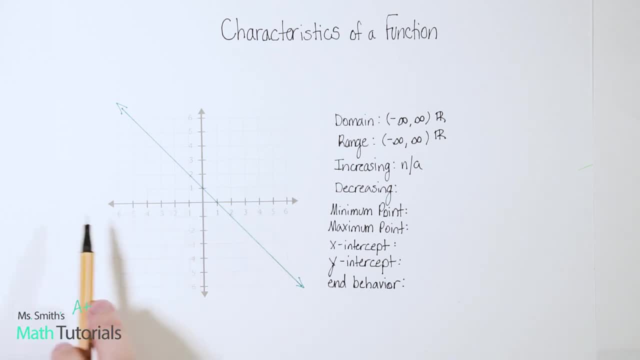 the x-axis, it would be negative infinity because it's going to the left. So remember, infinities always get parentheses. Negative infinity. and then, for how long is it decreasing? Well, it's going to be for the entirety of this line's life. Okay, all the way to positive infinity. 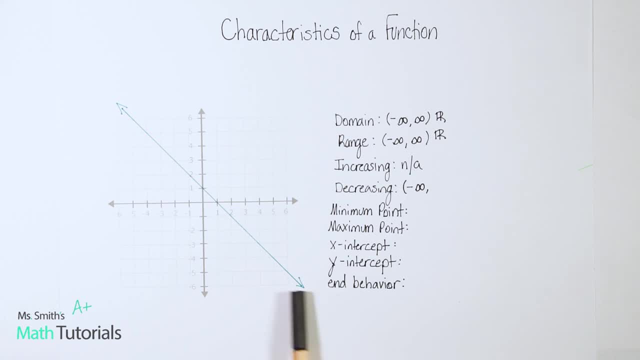 and some people might say: but that's going down. Well, it's going down on the y-axis, On the x-axis it's going up. So we call that positive infinity. So this graph is decreasing from the interval of negative infinity to positive infinity. Our next thing we need to be able to pick out is if there 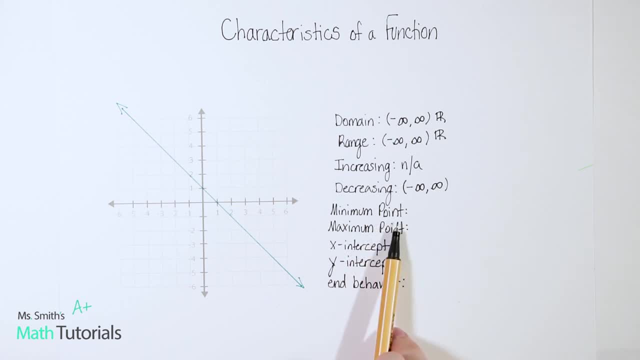 is a minimum point And the key word there is point Now on your tests or quizzes or homework. it doesn't always write point but it's assumed. So if it asks for minimum, you just think minimum point. Ask yourself, is there a lowest place on the graph where this line will stop? And that is the lowest point, the minimum. 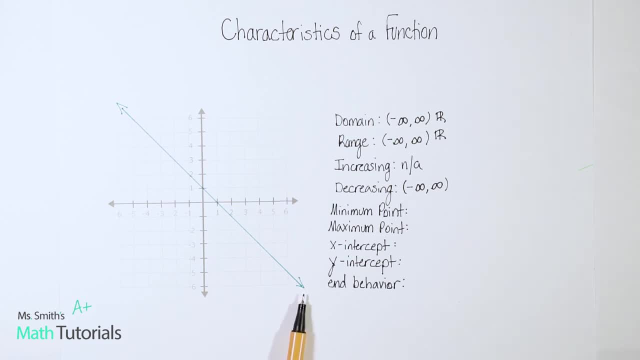 point And the answer is no. I see this arrow and I know that this graph is going to go on down for infinity, so there is no minimum point. There is no minimum point that I can pinpoint. Some people would want to say: well, infinity is. 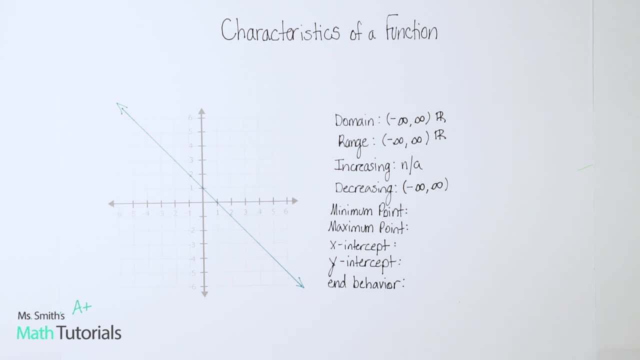 a point. Well, no, infinity is just an expression that means it goes on forever. It's not an actual point In this case. a lot of that to say there is none N-A or none. Is there a maximum point that I can, that I can literally point to and say that is as high as the graph goes and it? 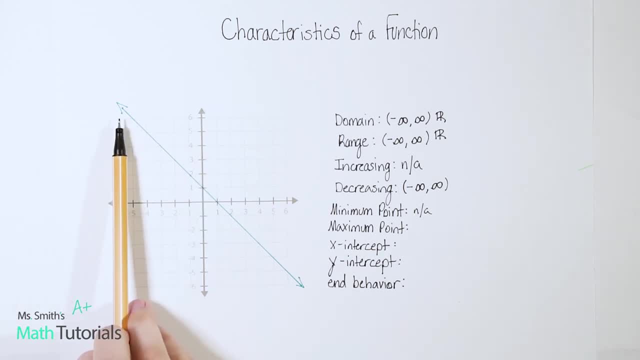 will never go beyond that point. No, This graph as far as height is going to go up towards infinity. Again, we got a lot of N-As on this one X-intercept- finally something we can answer. So we want to know where does this graph cross the x-axis? And it may happen at nowhere, It may happen at multiple. 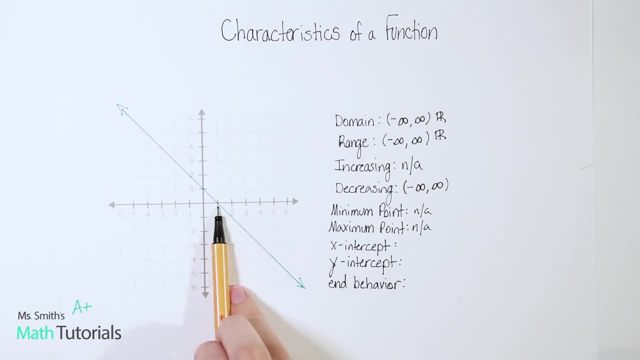 places. In this case it only happens once. We see right there now, different teachers have different preferences of how they want you to write the x-intercept. I prefer just for you to write the actual point. I like to write the x-intercept right there at that point and that point falls at one zero. So I 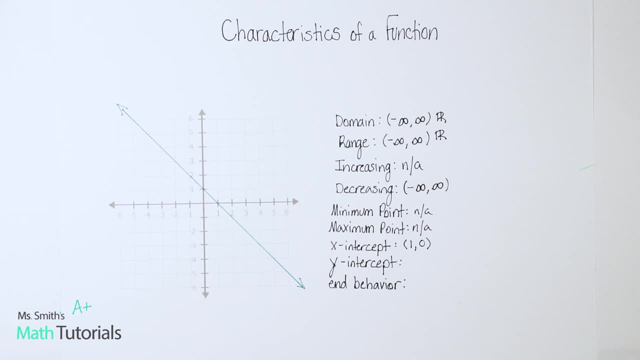 like to write that point as one zero For our y-intercept. So now we're looking at where does this line cross the y-axis, and I see it happens right there, And so I want to list out that point full point as well, and that's at zero positive one. 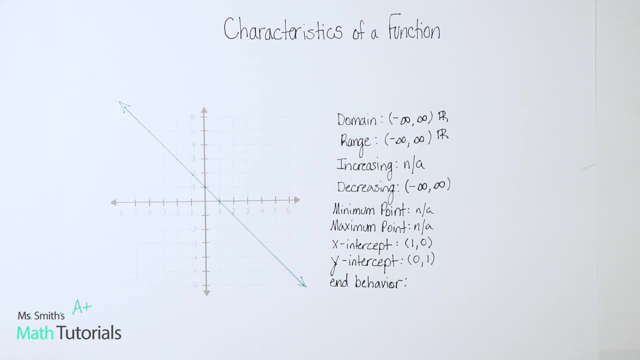 Now, end behavior is kind of interesting. End behavior is a phrase that you really need to memorize. Sometimes teachers will give this to you and it's like a fill in the blank format, and sometimes they're just going to expect you to write the entire end behavior. 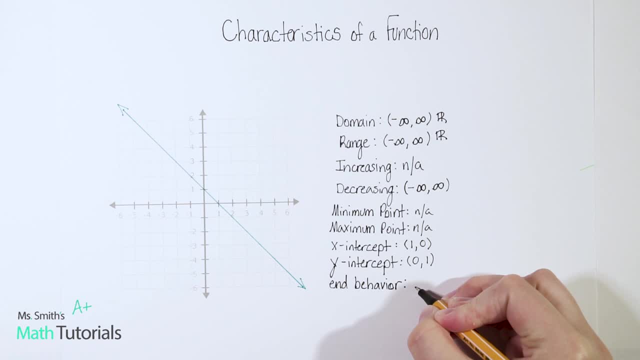 So you really need to memorize it. As x approaches- That's what that arrow means- approaches As x approaches negative infinity. As y approaches- And this is what we have to think about. So let's think about that- As x approaches negative infinity. Well, if this is our origin and we're talking about the x, 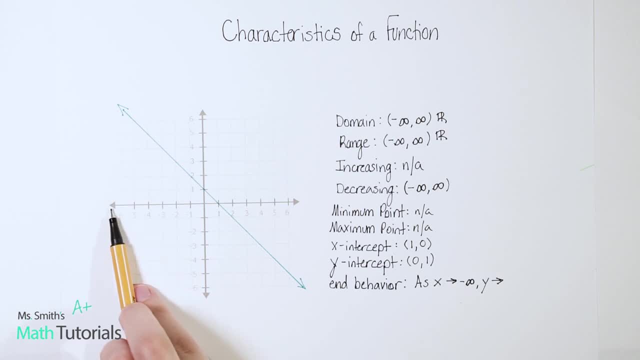 As x goes this way, because that's towards negative infinity on the x-axis, We have to ask ourselves: what is y doing, What is that line doing? And typically your answers are going to be: it's either going up, It's going down. 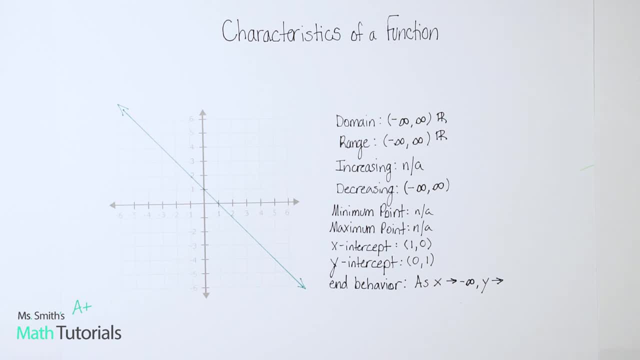 leveling off, sometimes like going in a straight line to the left. In this case it's going up and the way we note that in n behavior is positive infinity. It's going up towards positive infinity. So, as we read this, as X approaches negative infinity, Y approaches positive infinity. But then we have to have a second. 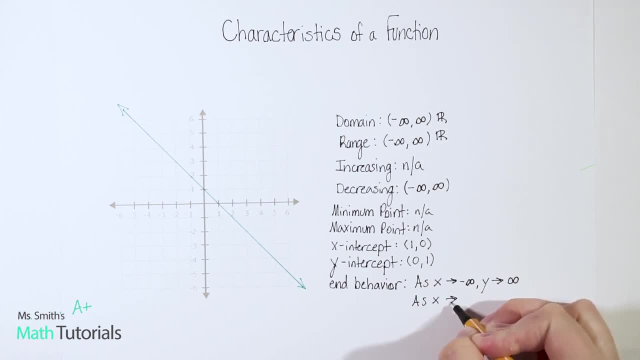 statement that, as X approaches positive infinity, what happens to the Y? Y approaches what? So in this case, now we're starting back at the origin and we're saying: as x goes this way, as x approaches positive infinity, what's happening to my arrow, My blue arrow, in this case? Well, it's either going to be: 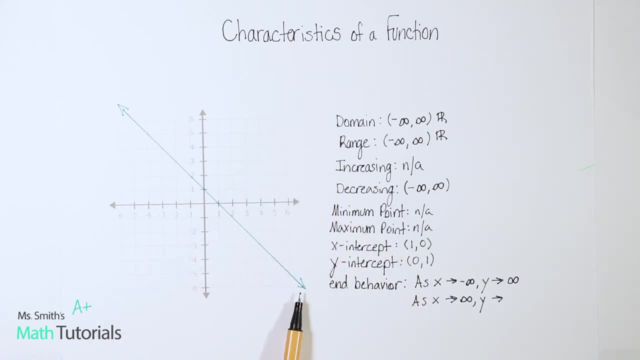 going up, going down or leveling off, and in this case it's going down. So down means negative infinity, negative infinity. So those are the statements. So sometimes teachers will just leave this part blank and they want you to fill in the endings, because this right here from the as all the way. 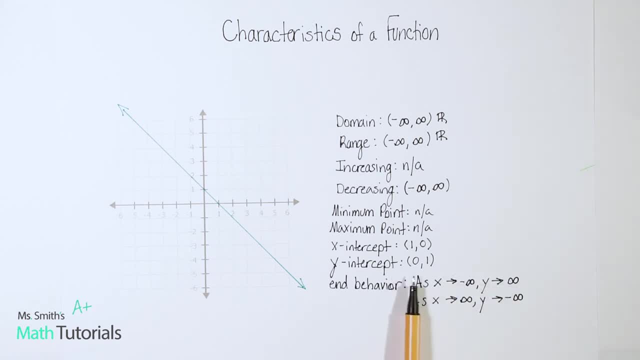 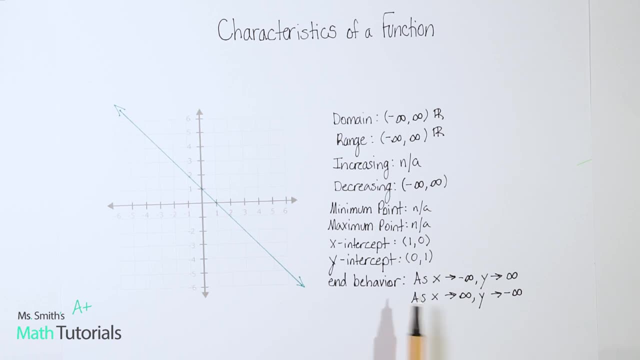 to the y approaches. that does not change. That statement stays the exact same every single time. These two little endings are what changes. but I'm gonna say, go ahead, memorize the whole thing so that you can be able to write it out if you need to. Let's look at some more examples. 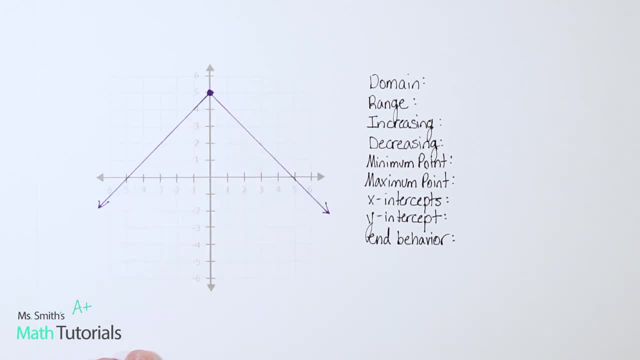 Looking at this graph, this is actually an absolute value graph. Don't need to know that right now. We'll get into that more later, but it's a good thing to know For our domain. remember domain left to right, in this case, negative infinity to positive infinity. 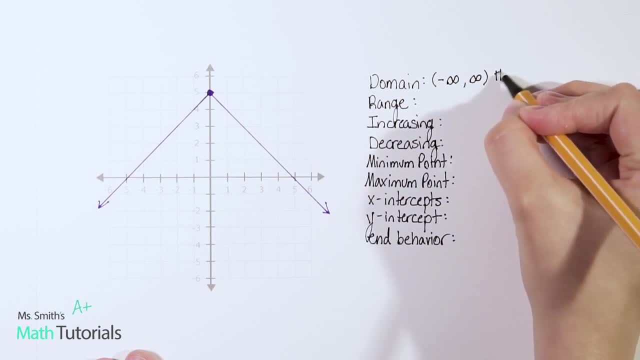 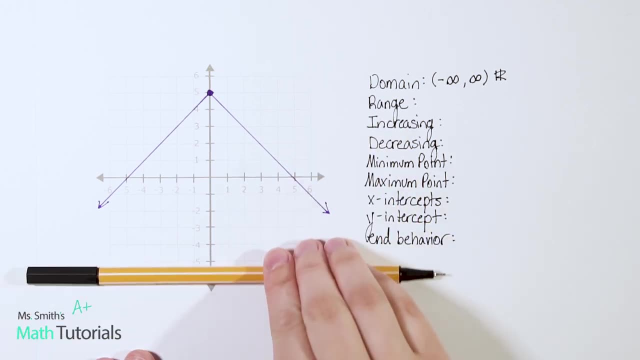 And remember, if you want a fancy way to write that double line R, We'll know what you mean For range: remember bottom to top. So in this case the first thing I hit is arrows. Remember arrows. indicate at the bottom, indicate negative. 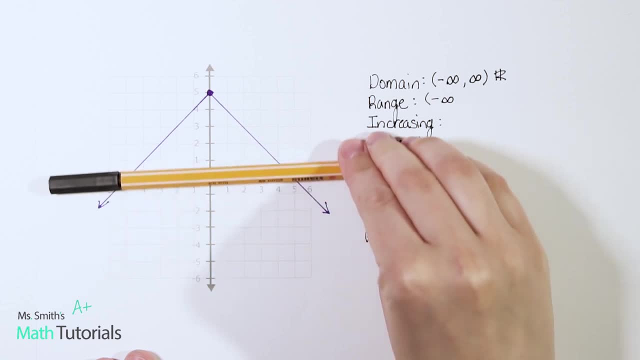 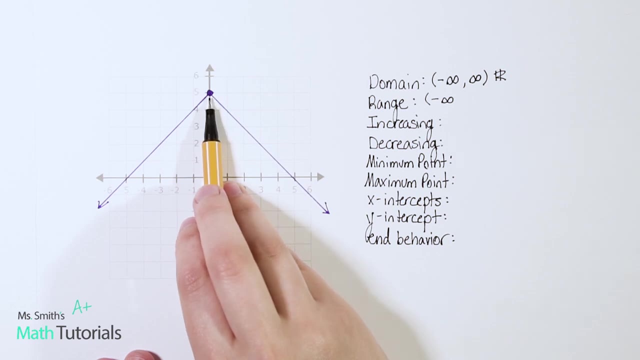 infinity. And then what's the top thing or the last thing that we hit? Well, this is actually a point, So it falls. it is a solid point, which means it's going to get a bracket and it falls at positive five. Range is talking about the y. 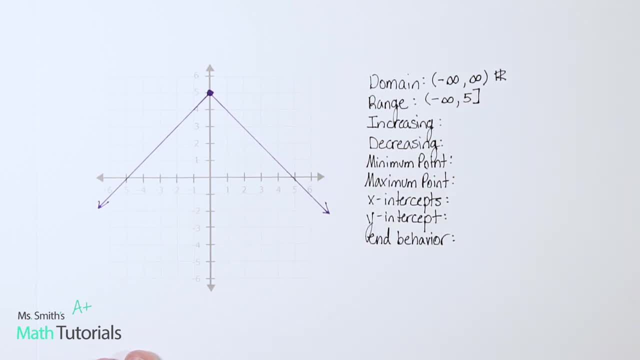 So five with a bracket. We could not do all real numbers on that. That's only if it's the double infinity Okay. As far as increasing and decreasing, well, I've got to look at each graph individually In this case. remember, we read it left to right. So here we see that we 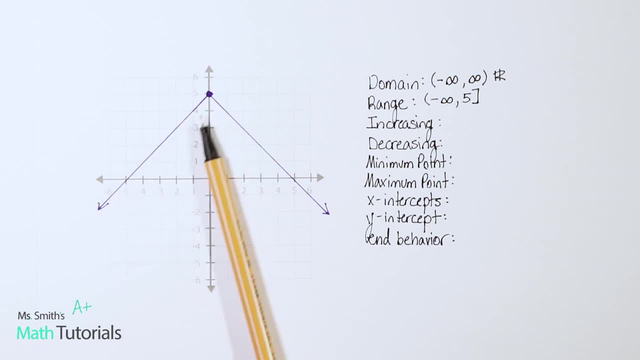 are increasing on this section right here. It's kind of like going up the roller coaster And then from here on down we're decreasing. So we're increasing on this section right here, And then we're decreasing. We're going down the roller coaster, So we do have both an increasing and 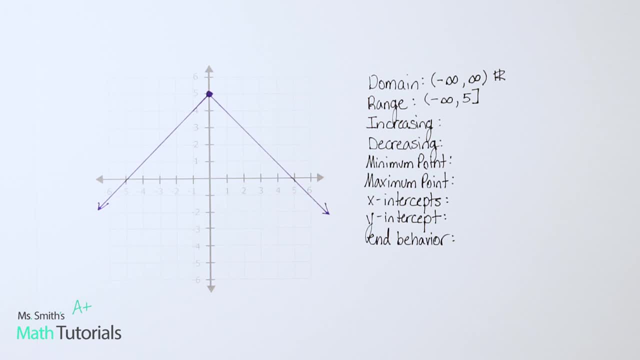 decreasing on this graph And we need to state what both of those are: The interval of x for the increasing and the decreasing. So let's start with increasing first. So it's a stretch from here all the way up to here. We're going up, So we start with. we always read left to right. We. 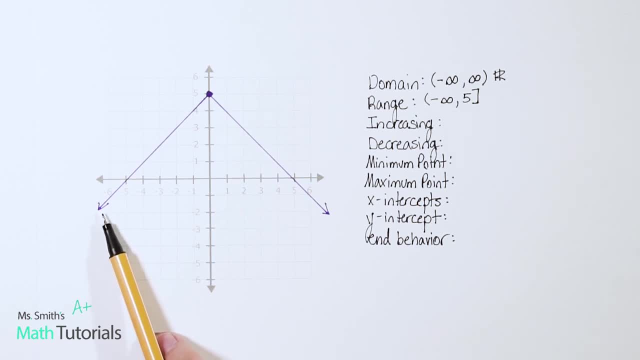 start with an arrow. Remember. arrow indicates- hopefully you're saying- negative infinity. Now, when we move up here we'd want to say on the x-axis. Remember I said on the other graph we are only talking about x values with increasing and decreasing, I do not care. 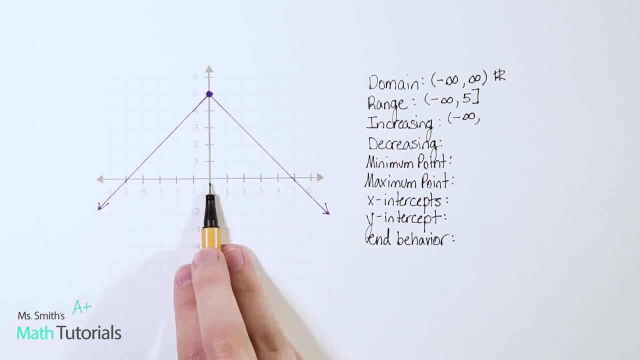 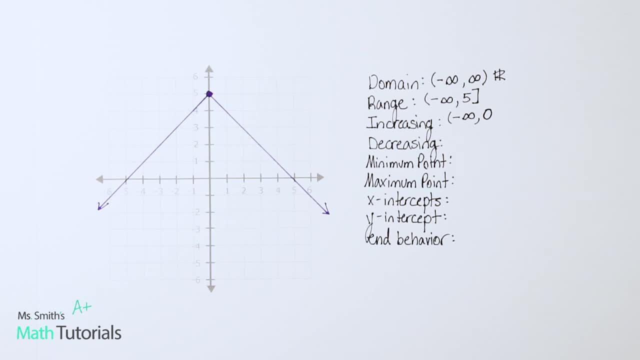 able to do that. I should have a zero with a bracket. The weird thing about increasing and decreasing is you have to ask yourself a question: Is this point a place of change? And what I mean by the place of change is: does it switch directions right at that point? In this case, I'm kind of 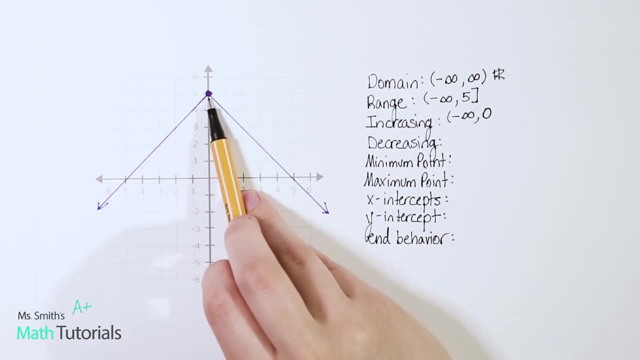 going straight, going straight, going straight. And then, when I hit this point where it also stops increasing, it switches and it goes down. So because we call that a place of change, it automatically gets a parenthesis, Even though it's a solid point, and you want to put a bracket. 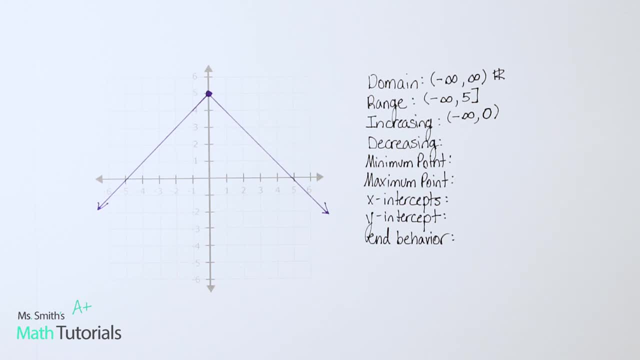 it's actually a parenthesis. So that is the trickiest part about increasing and decreasing is remembering that. So let's do decreasing now. So I'm decreasing from here to here, from this interval to this interval, or from that interval of time from here to here. So 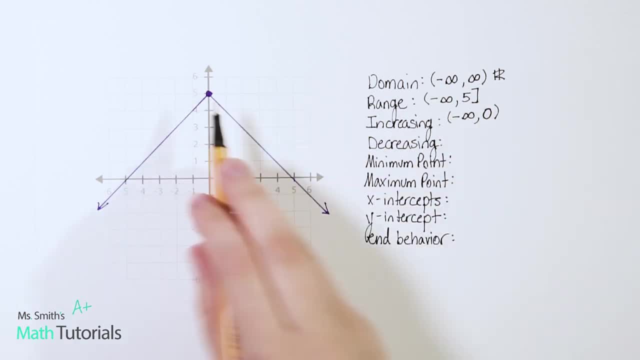 it goes from zero And remember it's a place of change, So that zero gets a parenthesis And it's decreasing all the way to positive infinity, Even though it's going down. we're looking at our x values: okay, And the x values are going this way and that's positive. 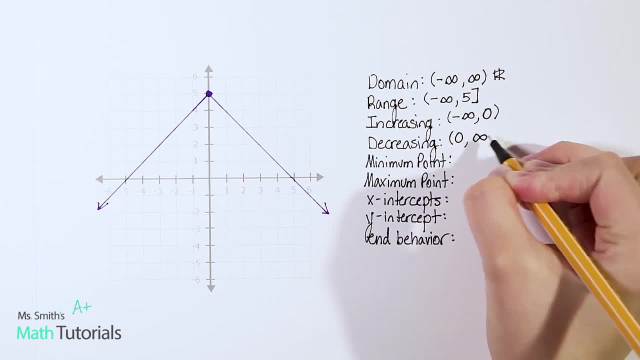 infinity, And I mentioned this in my other video. You will never have a negative infinity on this side. You will never have a positive infinity on this side. If it's on the left, it's negative. If it's on the right, it's negative. If it's on the left, it's negative If it's on the left. 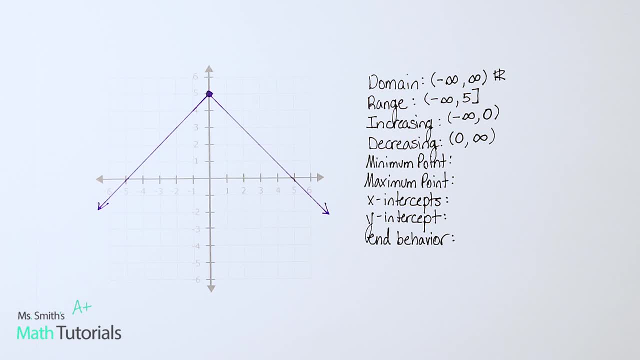 it's on the right, it's positive. So that may help you remember. Okay, let's move on to minimum point. Is there a lowest point on this graph that I can literally pinpoint and say that's as low as the graph goes and it doesn't go any further? And look, some people would say, well, there's that. 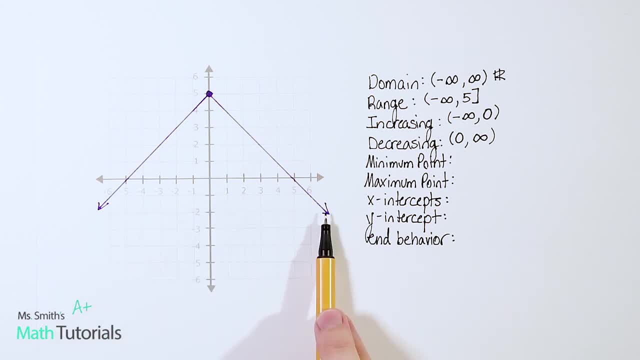 point, or there's that point. Well, those aren't points, Those are arrows. okay, So they're going to keep going on forever. So is there a minimum point? Nope, You will never have infinity as a minimum or maximum. And now maximum point We do right up here, This graph will never go above positive five. So we 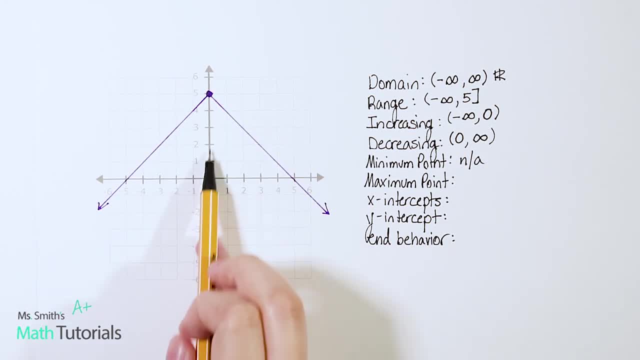 want to actually list that point. So it falls at zero. positive five Our x-intercepts. we've got two here, I've got one right here and one approximately right there. We'll say that that's positive five. I'm going to go ahead and do this, So give me a little grace right there. So I need to list both of. 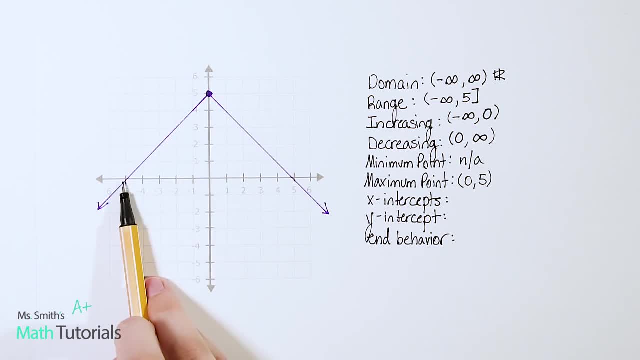 these individually. So first let's say this falls at negative five zero, And because we do have a second one over here, positive five zero For our y-intercept, we just have the one right up here, that point again.